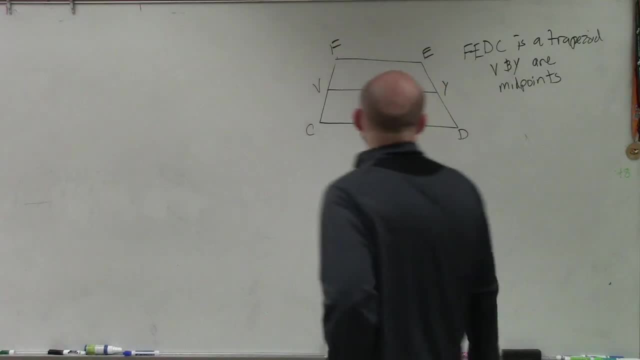 So, on this case, you guys have FEDC as a trapezoid, where V and Y are midpoints. So if we know it's a trapezoid, what do we talk about? What does a trapezoid have? 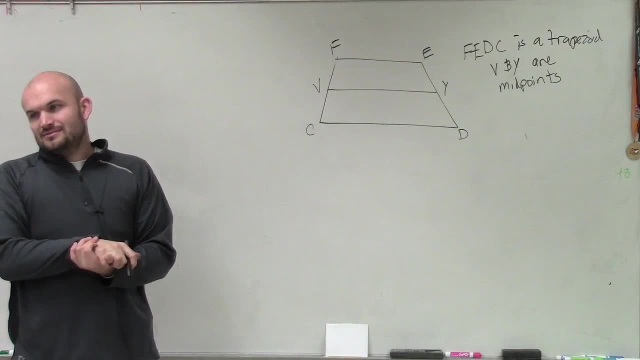 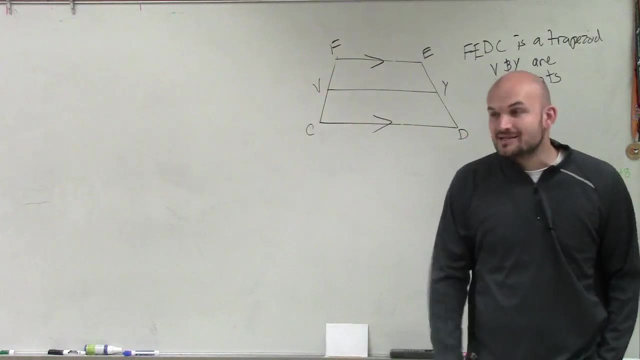 Aiden, what is one thing you know about a trapezoid? They have two parallel sides. Yes, Aiden, you have a really high voice. Yes, very good, They have a set of parallel sides right Now. the next thing is- they talked about this midpoint- that V and Y are midpoints. 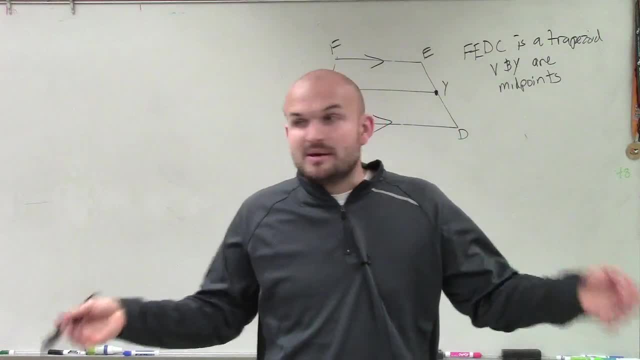 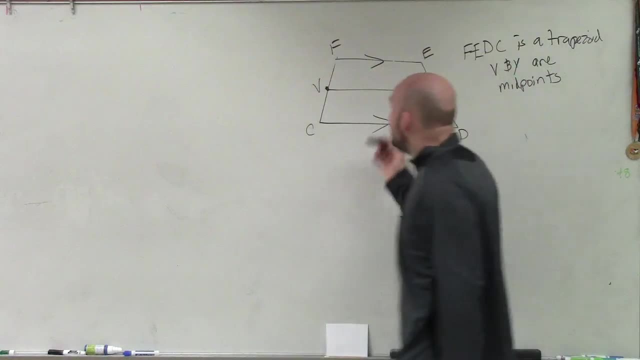 Now, if you guys remember the midpoint created, if you have your two midpoints and you connect them, those what they did, Keith, those created what we call the midsegment, And that midsegment is also parallel to. these are what we call our two bases. okay, 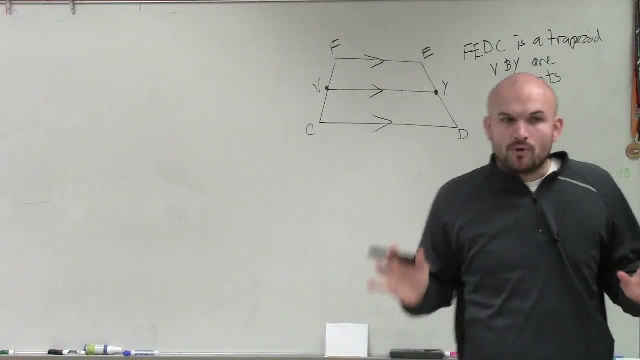 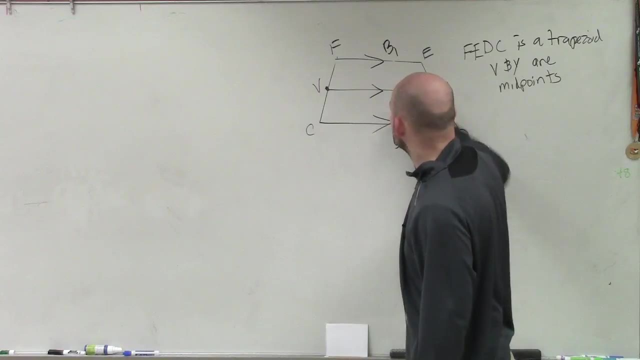 And this is pretty much what you missed last time- our two bases. Now, what was really important about this was: there is a formula for all this. right, If I called this base one and this base two and this the midsegment, do you guys remember? 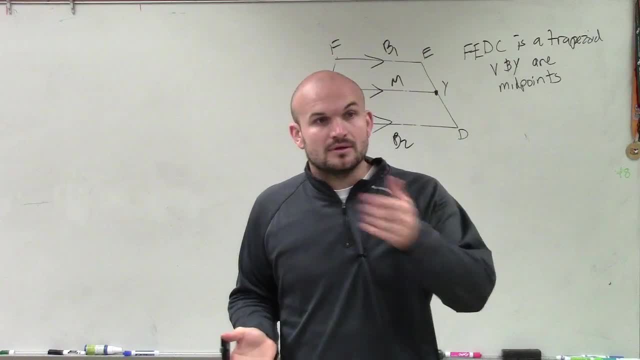 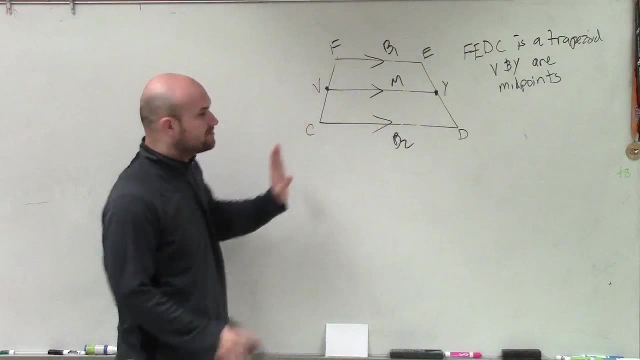 There is a formula for how these lengths were connected, right? Yes, Well, you're going to have one for that particular problem, right, Yeah, but that's all right, So I'm just going to use this. So what we had was what we talked about was our midsegment, which I'll call M in this case. 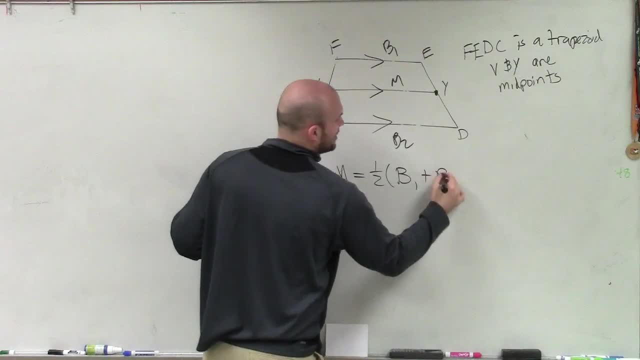 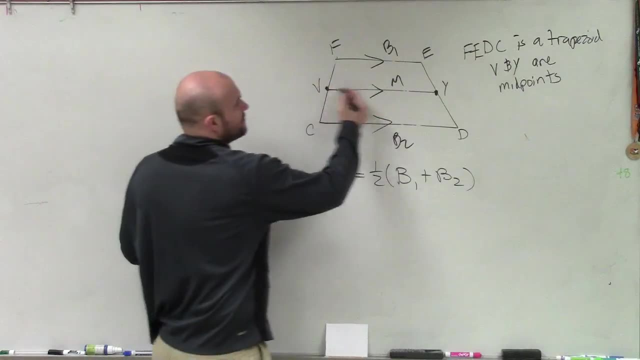 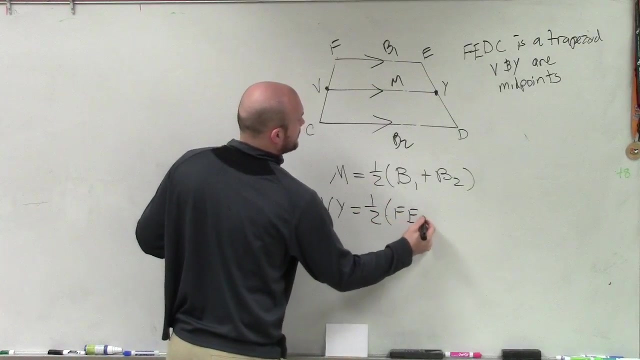 is equal to one-half base one plus base two. Well, I don't want to use M's and B's and H's. How does it relate to this problem? V? Y is congruent to one-half F, F, E plus C, D, right? 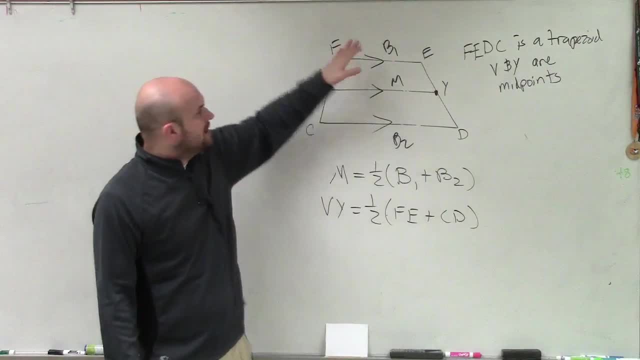 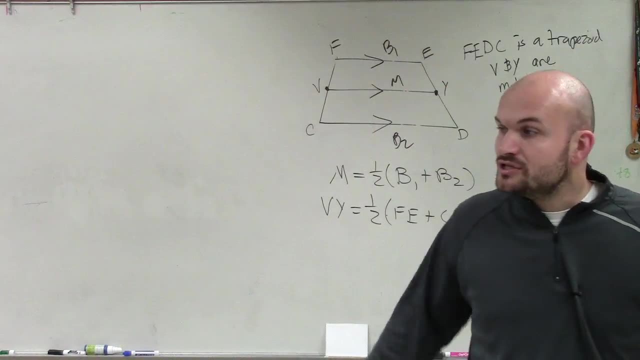 Where M represents midsegment, B represents base one, base two, but I'm actually labeling them how they are in this problem. Now it's important. This is number six. Now, what's important about this one is we actually know some of these lengths. 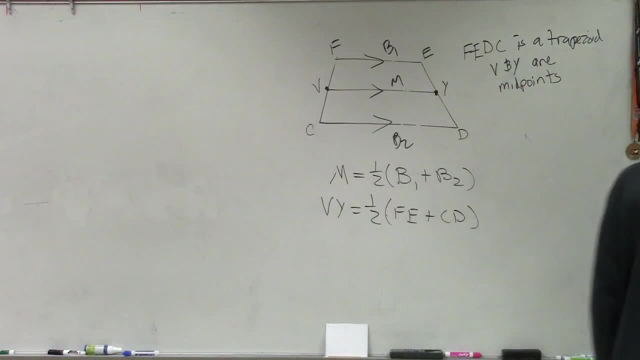 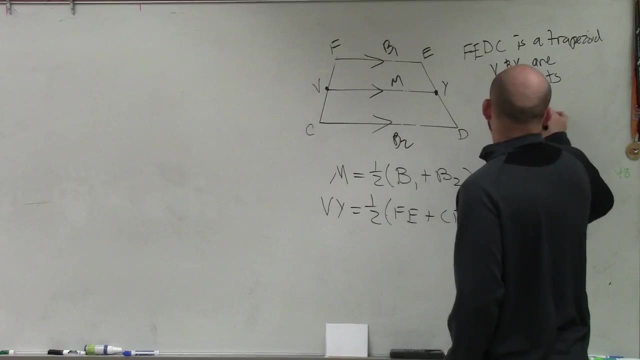 So you guys can see: oh, we don't. We do know, but I just didn't write them down For six. no, I'm sorry, this is five. It says F? E. F- E equals 18, and V? Y equals 28..